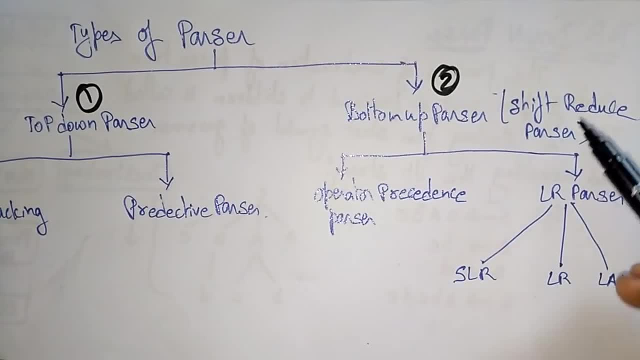 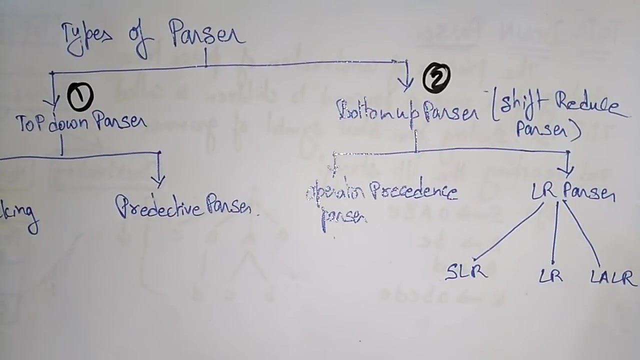 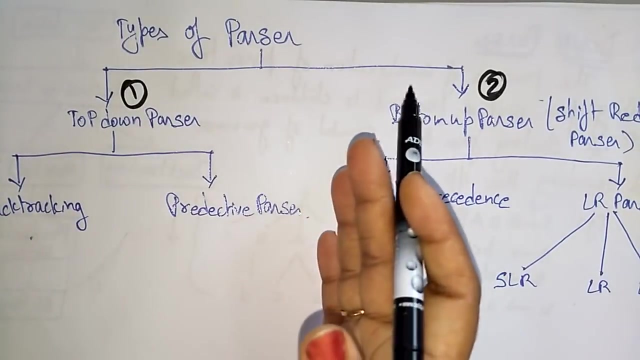 Top down parsers, whereas bottom up parser is also called, as a chef, bread juice parser. So this bottom up parser is of two types. One is an operator presence parser, LR parser, again LR parser- of different types: SLR, LR, LALR, CLR. Okay, so these are all the different types of parsers, So let's see one by one. First we'll discuss about the top down parser and what are the different types of top down parsers, what they are playing. 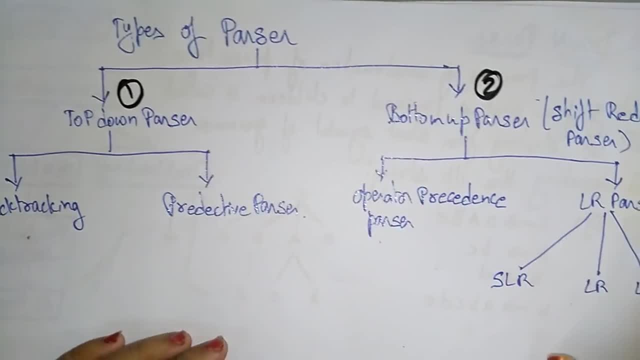 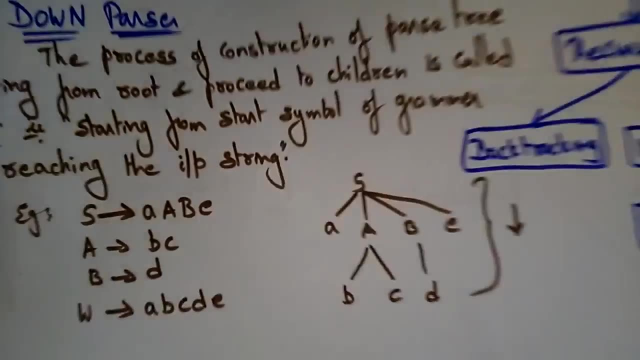 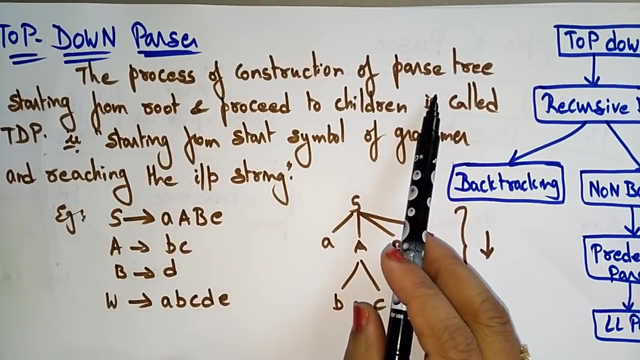 role in the syntax analysis. okay, and after that, bottom up, now let's see a top-down parser. top-down parser. the process of construction of parse tree, starting from root. okay, the process of construction of parse tree. okay, this is a tree, this is a parse tree, starting from the root. 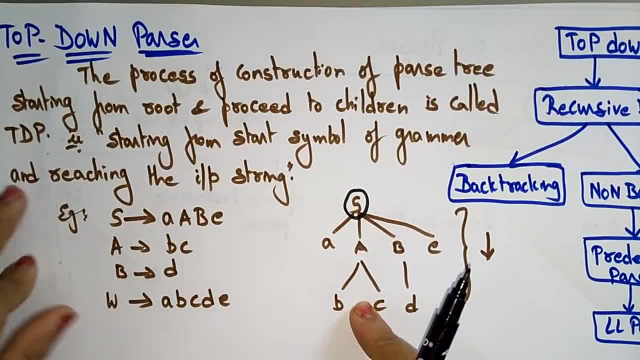 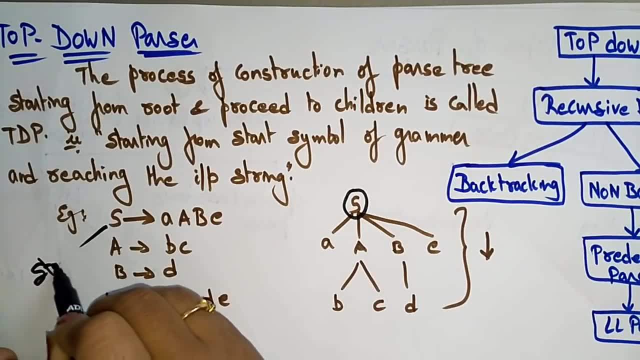 and proceed to children is called top-down parser. that means starting from the start symbol. so s is the start symbol, s is the start symbol. so this may be anything okay. so it, uh, there's non-terminal, maybe e, t, s, whatever it may be okay. so starting from the start symbol of a grammar. so this is a. 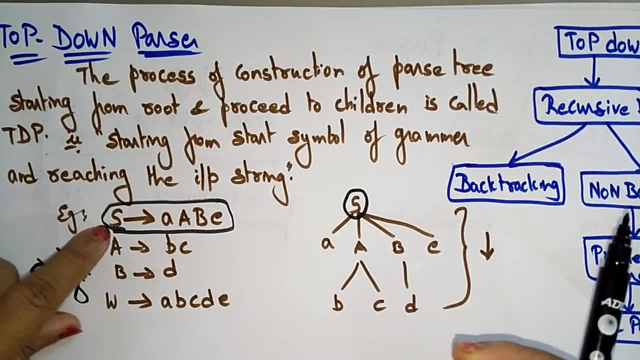 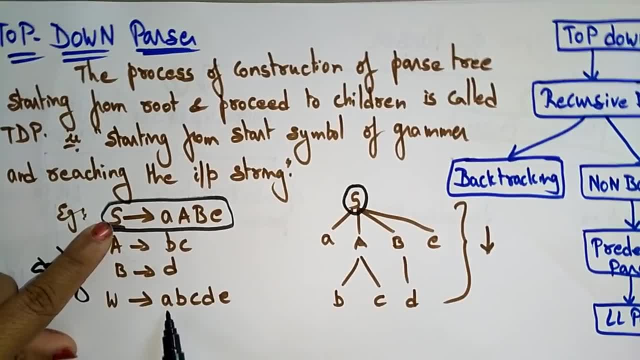 starting symbol of a grammar. whatever the grammar you are taking, that is a starting symbol, is this okay? this start with the starting symbol of a grammar and reaching the input string. so the final thing is we have to reach the input string. so what is the input string here? w is equal to a, b, c, d. 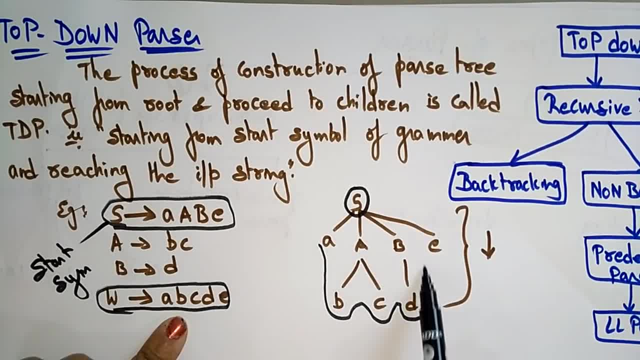 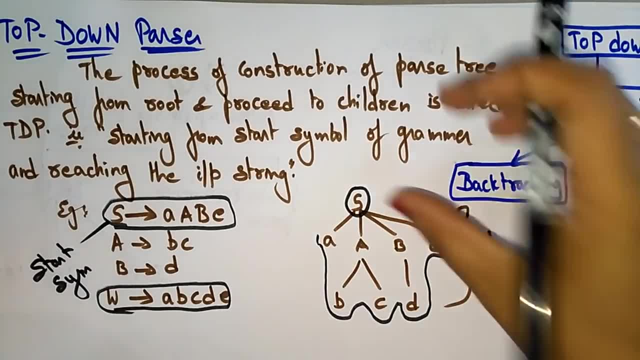 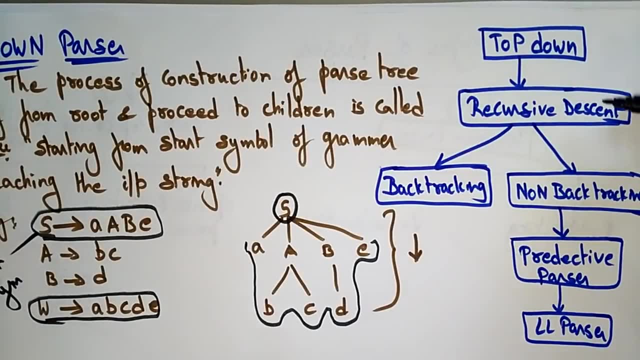 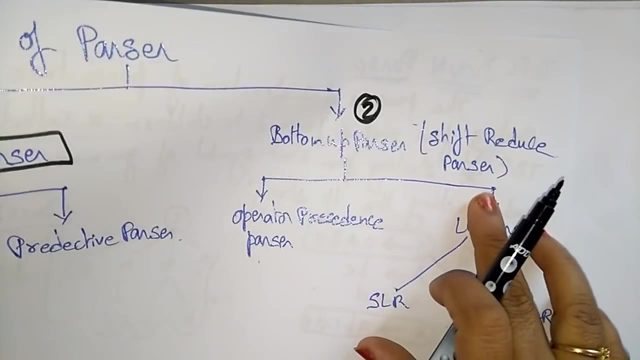 so we reached the input string. this is the concept top-down. so from top to down you have to be scan, starting from the start symbol of a grammar and reaching the input string is a top-down parser. so the top-down parser is a recursive descendant parser. we call it as a, whereas the back, uh, bottom, of what i said it is a shift reduced parser. 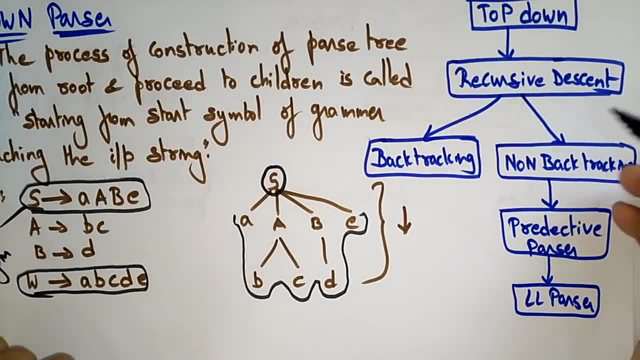 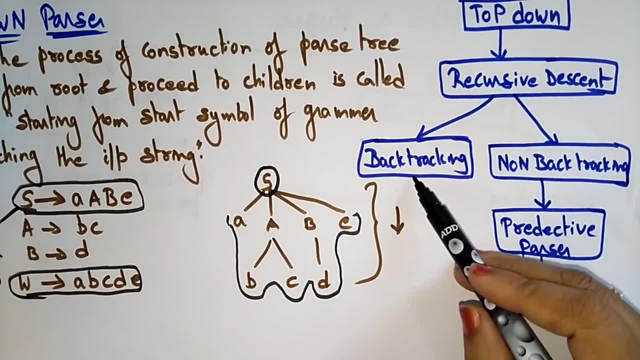 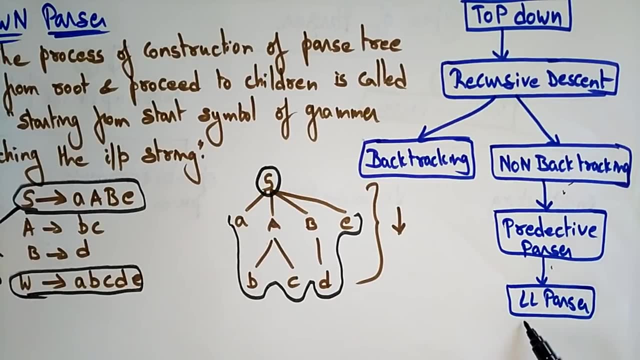 and whereas the top-down parser is a recursive descent, the recursive descent is a follow back tracking, a non-backtracking system. so the recursive descent may be backtracking or non-backtracking. non-backtracking comes under the predictive parser and again, the predictive parser is an example for the ll parser. the example is ll parser. so, with the help of ll parser, you are. 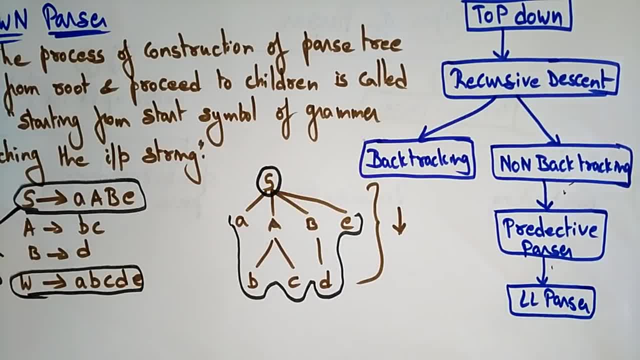 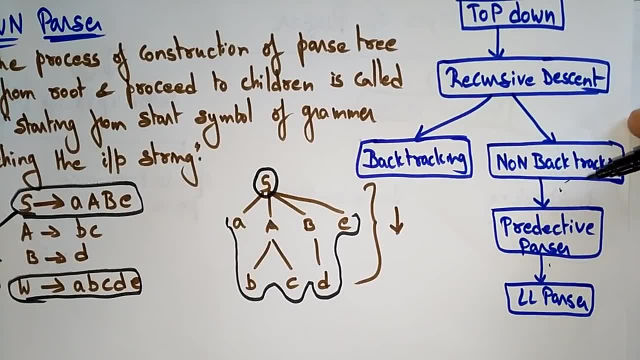 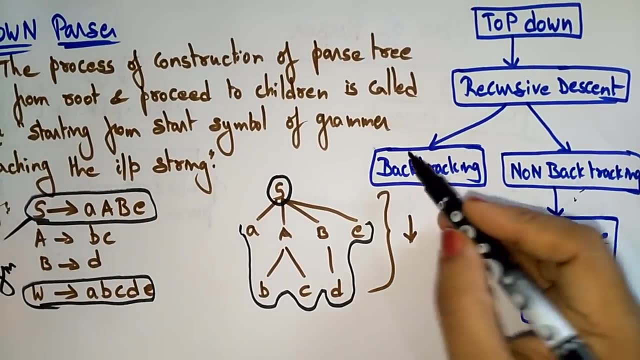 to solve this predictive parser. so top-down is a recursive descent. this recursive descent is of two types: backtracking and non-backtracking. the non-backtracking system comes under the predictive parser and ll parser. okay, so in this video i just want to explain what is a backtracking. 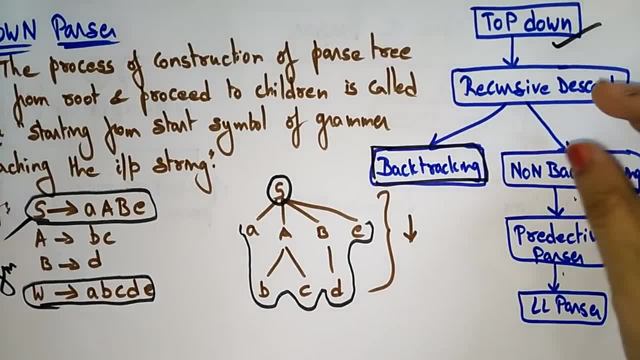 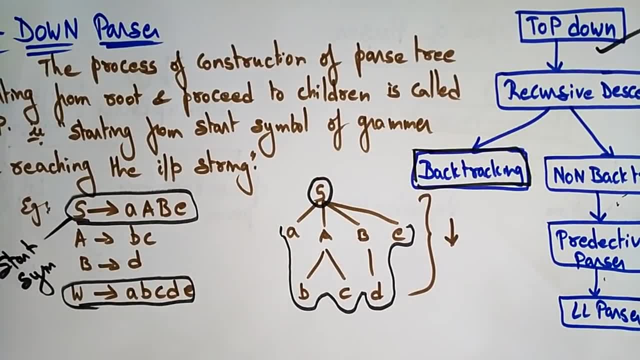 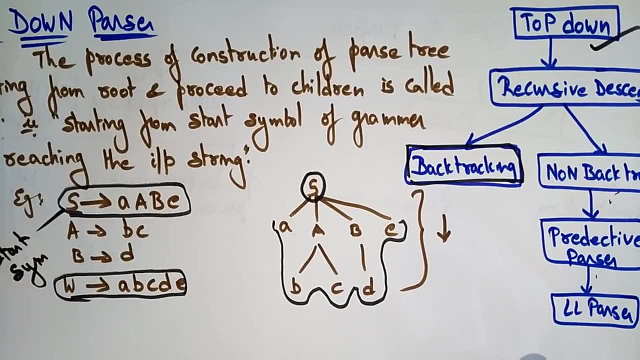 we are discussing the top-down parser, so the top-down parser will see what is a backtracking. so here you the thing you have to be. no, uh, note on that in the top-down parser internally uses leftmost derivation. the main concept here is: uses the leftmost derivation. 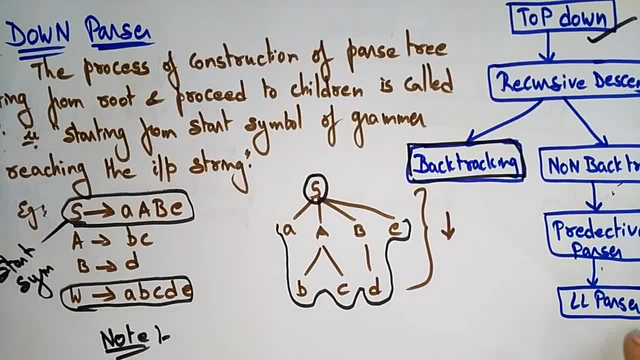 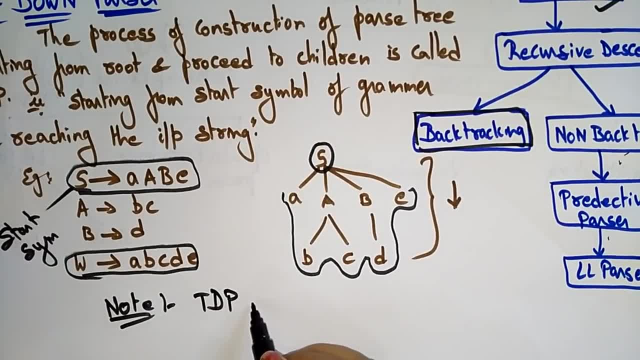 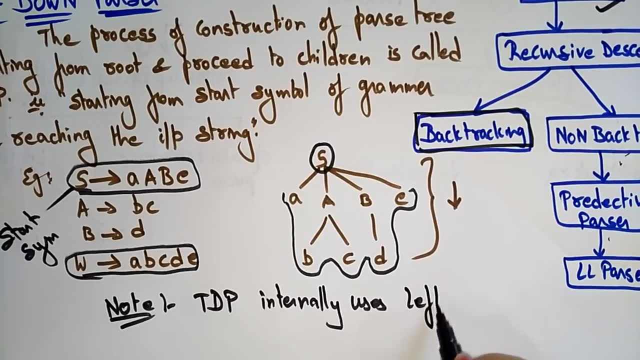 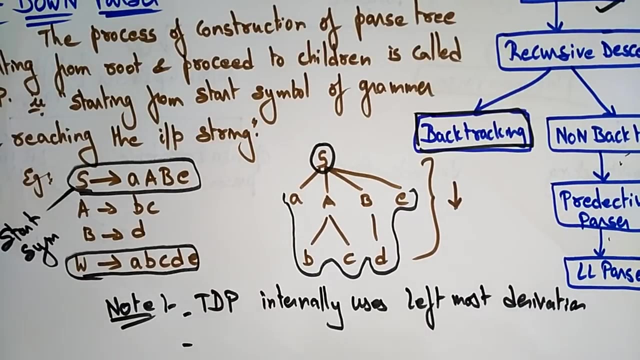 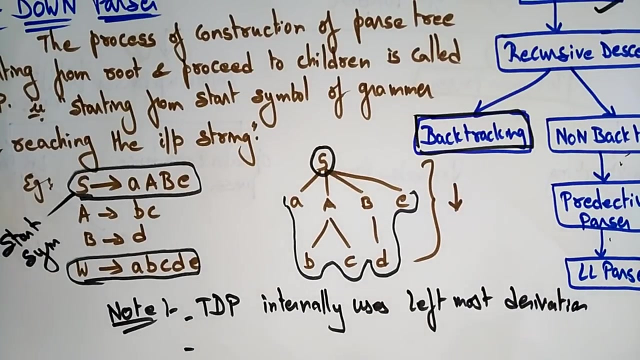 so let's discuss the top-down parser in clearly with brief points. later we will see the back tracking. the top-down parser internally uses- internally uses left-most derivation. so left-most derivation, okay, it uses the leftmost derivation and top-down parser constructed the constructive further grammar, if it is a free from ambiguity. 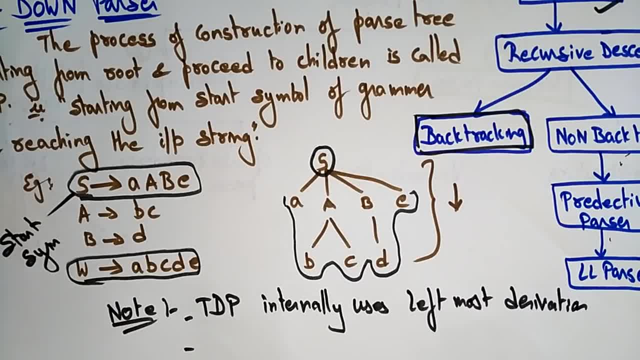 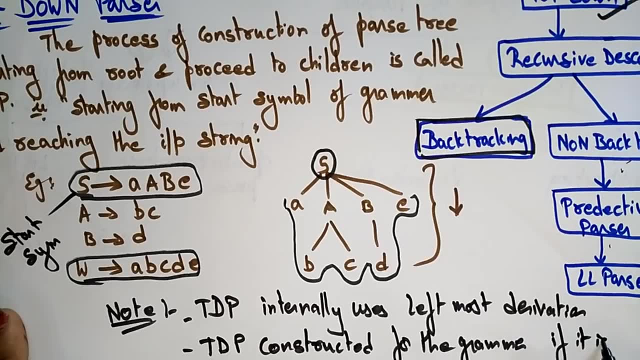 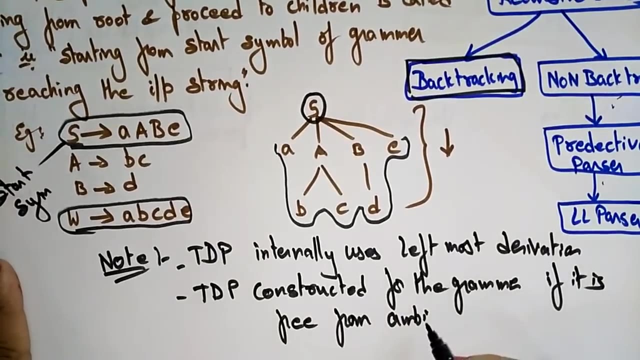 and left recursion. so when you construct the top-down parser, so this top-down parser constructed. it is constructed for the grammar for which grammar it will be constructed? grammar if it is free from ambiguity, free from ambiguity and left recursion. so when that grammar is free from ambiguity and the left recursion, then only the top-down parser will be. 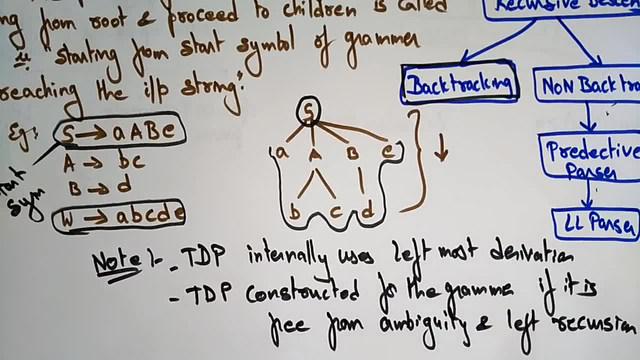 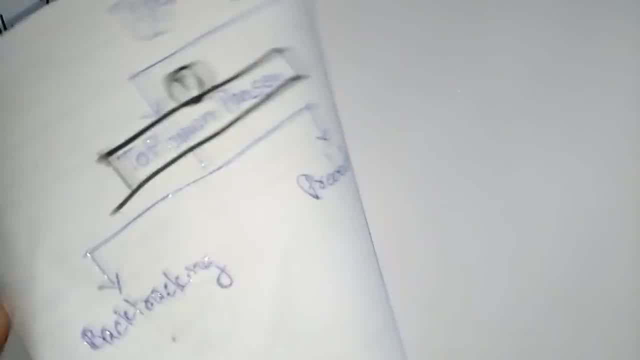 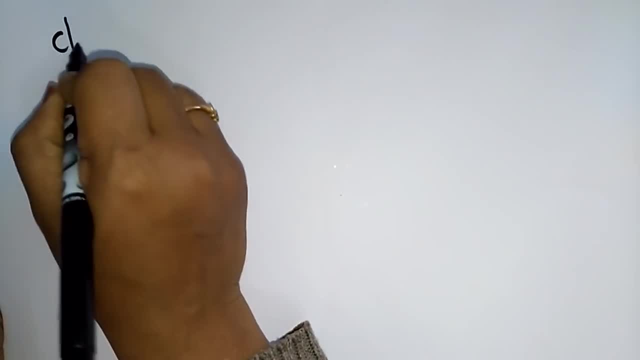 constructed. if there is no ambiguity in the tree, then we can construct the top-down parser. the average time complexity here is order of n square. okay, the different classifications of top-down parser is. let me directly. so still, we didn't enter into the different types of top-down parser we are discussing. 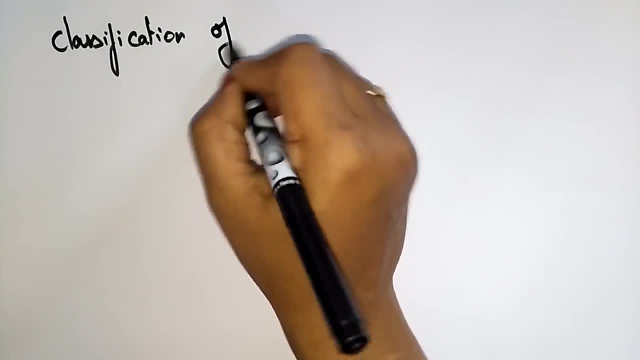 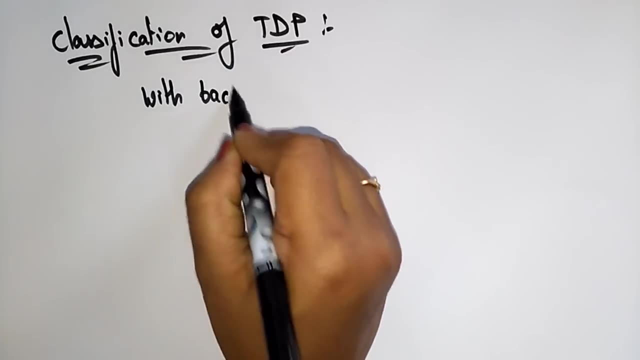 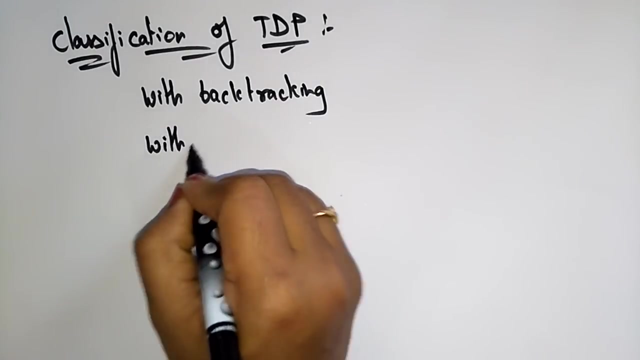 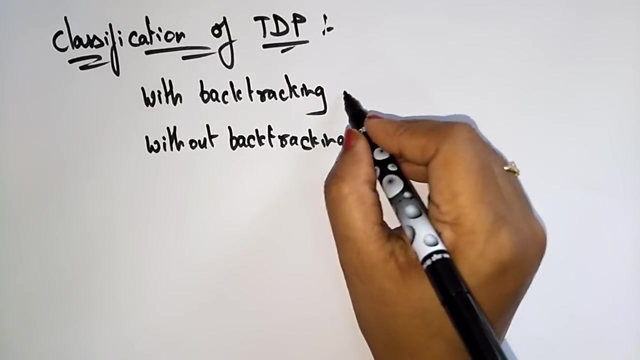 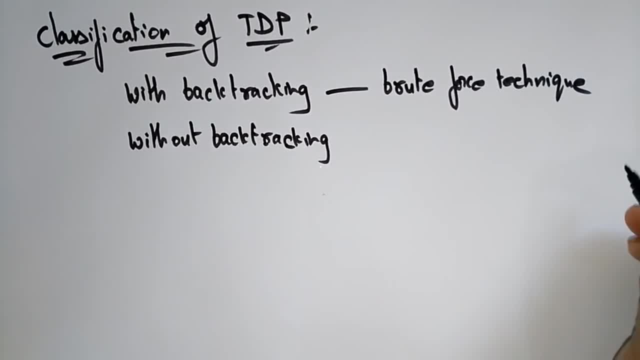 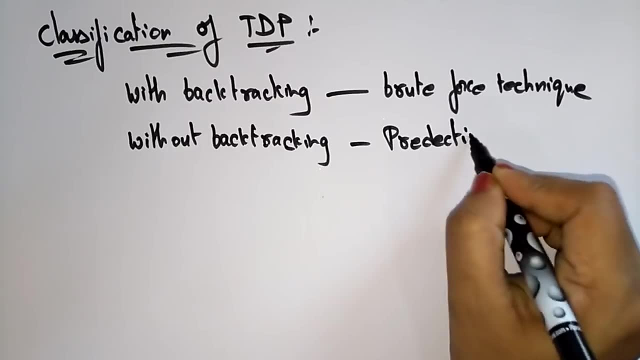 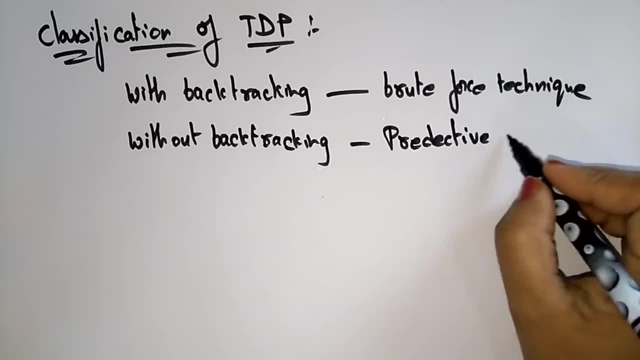 parser technique is a predictive. parser technique is a predictive. parser technique is a predictive parser. parser technique is a predictive. parser technique is a predictive. parser technique is a predictive without using the backtracking concept. predictive parser. okay again, this predictive parser is ll of one grammar. it uses ll of one grammar. 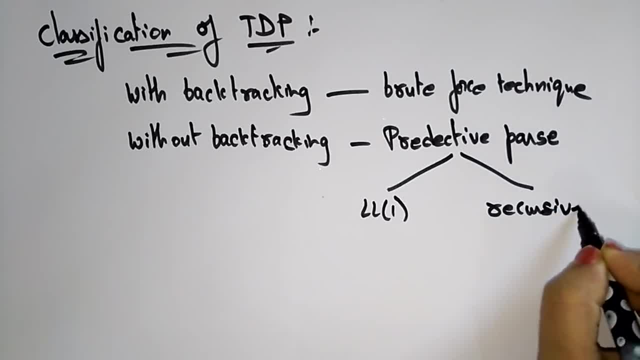 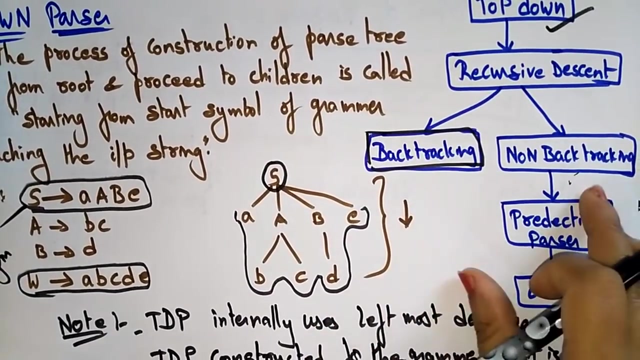 and recursive descent parser. okay, so this is about the classification of top down parser. uh, so let me clearly explain what is a recursive descent parser. recursive descent- okay. uh, here the recursive descent is of backtracking and non-backtracking. then both the concepts will use. so let's see what is a recursive descent. so up to now, what i 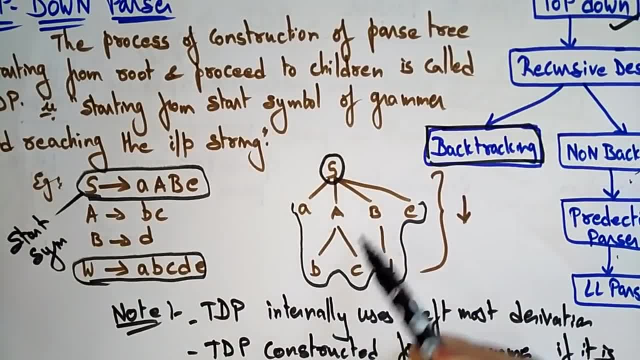 explained what is a top-down parser, how the grammar will be constructed. so, with the help of the grammar, by using the starting symbol, you need to parse the tree. okay, so s is a, b, c in place of a, just substitute b, c and in place of b, you substitute d. with the terminals, the non-terminals. 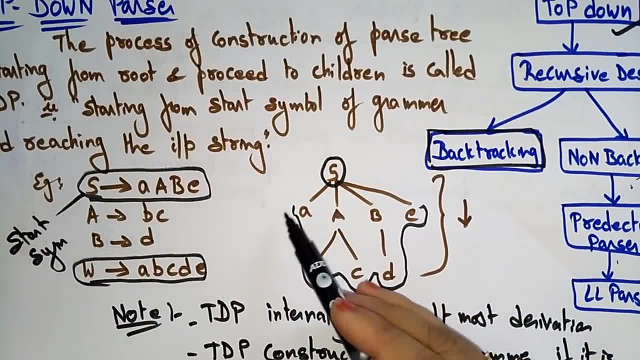 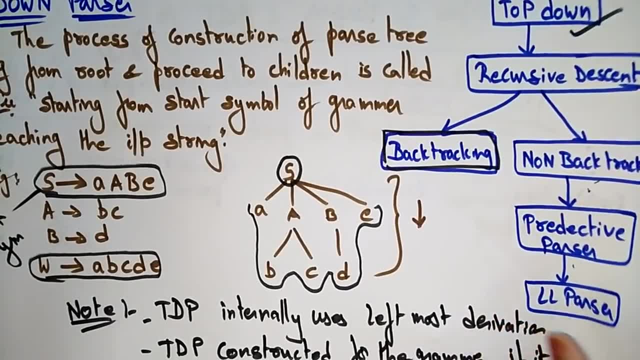 will be replaced with the terminals and you have- uh, you have- to follow the top-down process. so the top-down process is of two types: backtracking and non-backtracking. so it uses a recursive descent concept. now let's see what is a recursive descent. later we will see. 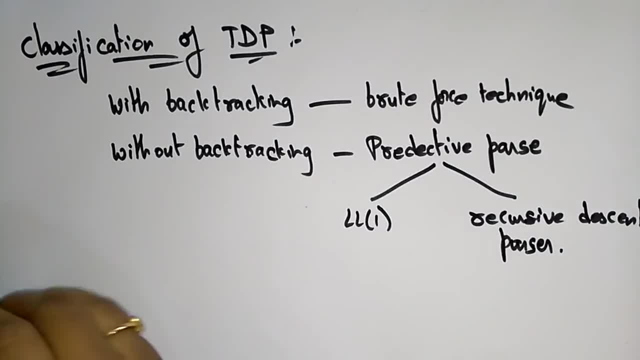 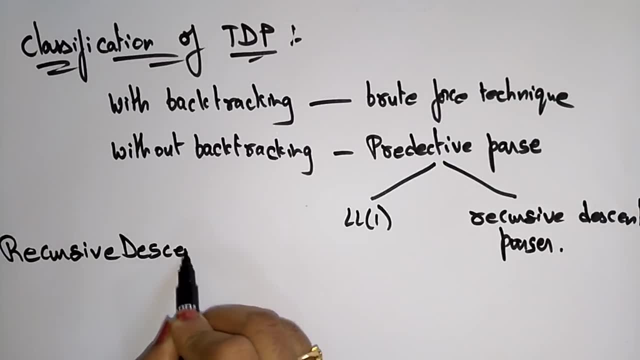 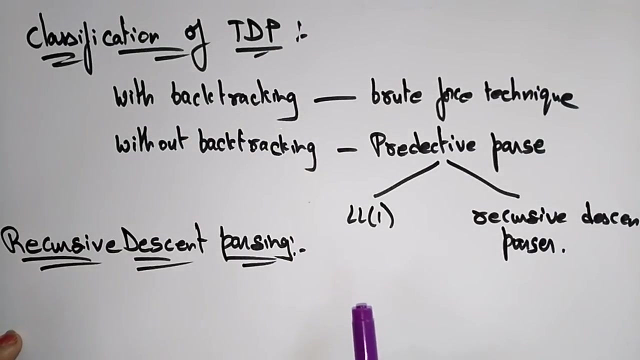 what is a backtracking and without backtracking technology, recursive descent parsing. so what is the recursive descent parsing? so actually, uh, under this technique, this recursive descent technique, the parser is constructed from top to down. so, because it is a top-down parsing, so it will come, the parse is connected from top to down and the input is read from left. 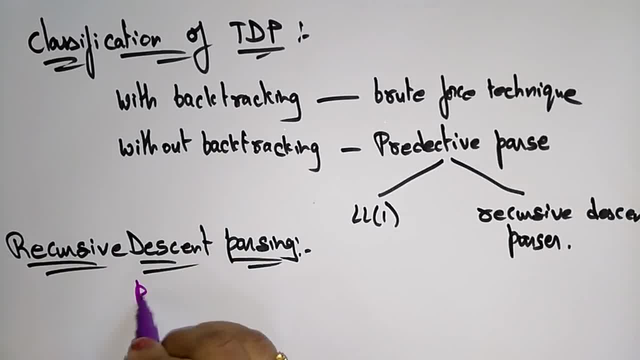 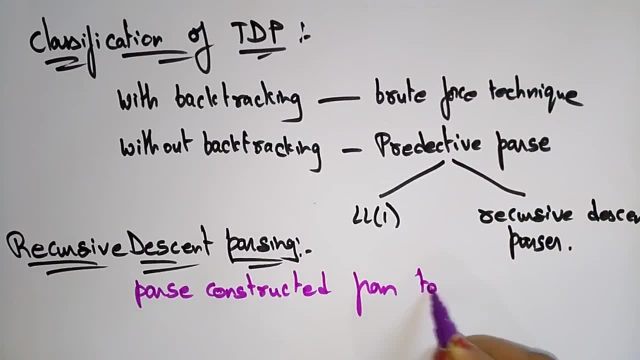 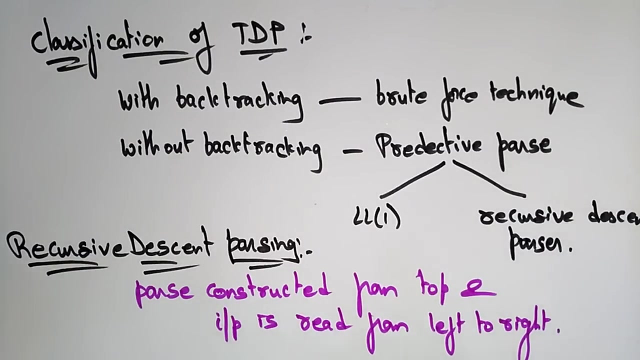 to right. okay, parse is constructed. parse is constructed from top stop and input is read from left to right. input is read from left to right, left to right. the input is read from recursive descent: the produces for every terminal. so, whatever the terminal, that is the produce. it produce for every terminal and non-terminal entity are used. so here the 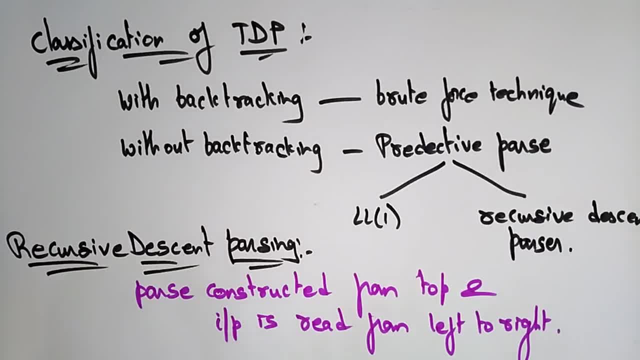 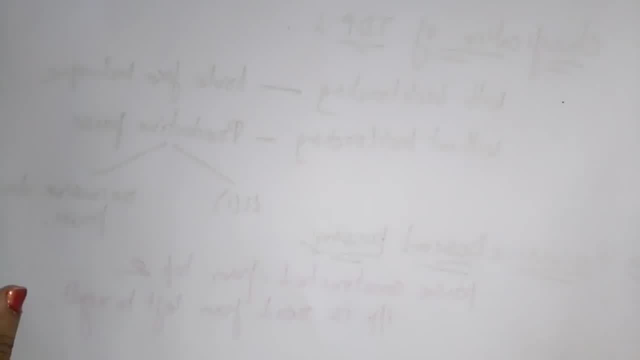 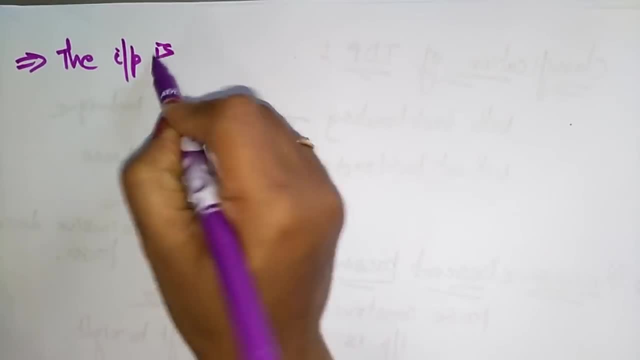 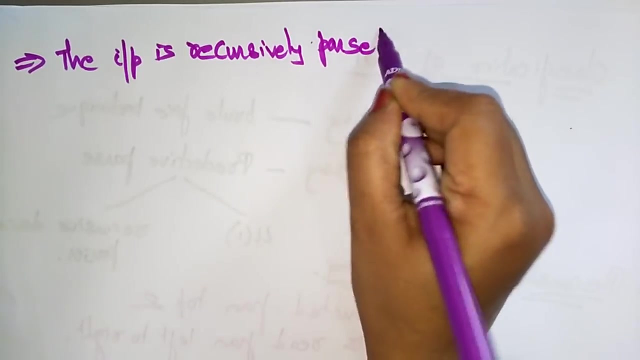 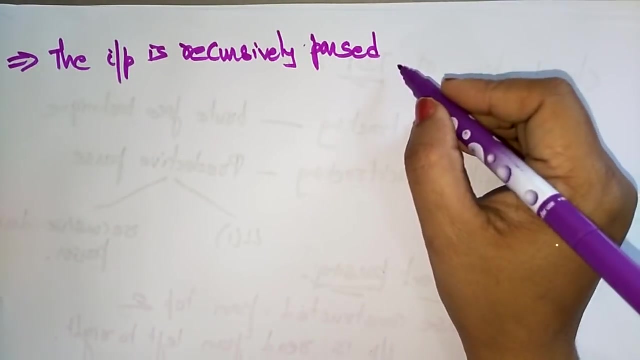 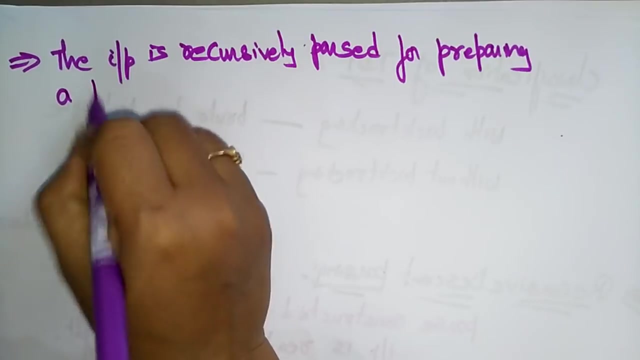 productions, whatever the productions are there. okay, for every terminal and non-terminal entities are used in recursive descent parsing. so here the input is recursively pursued. let me write that input is recursively parsed. so whatever the input that we are taking, so that input is recursively parsed. or by this technique, uh, for preparing a parse tree, for preparing a parse tree. so actually what we? 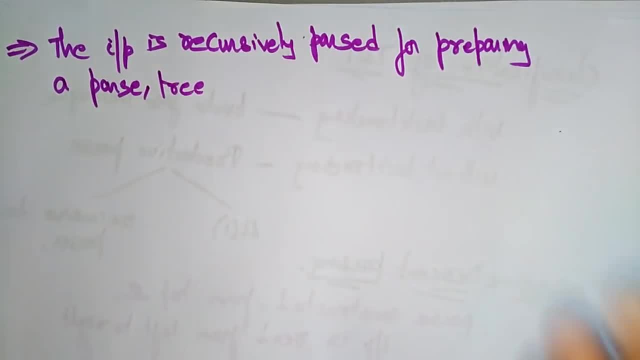 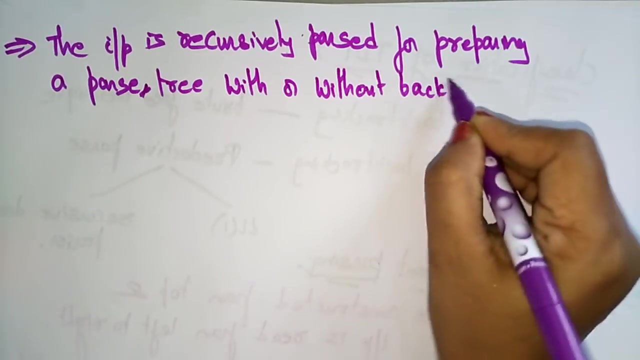 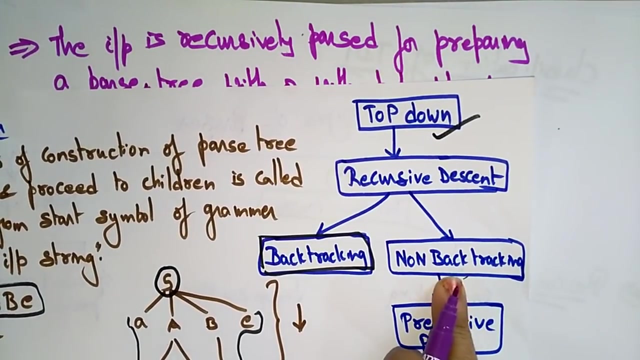 the aim of our recursive design. we have to construct the parse tree so the input is recursively parsed for preparing a parse tree, with or without backtracking, so it may follow, with or without backtracking, so that that is asset. the recursive descent may be a backtracking or non-backtracking, so it is. 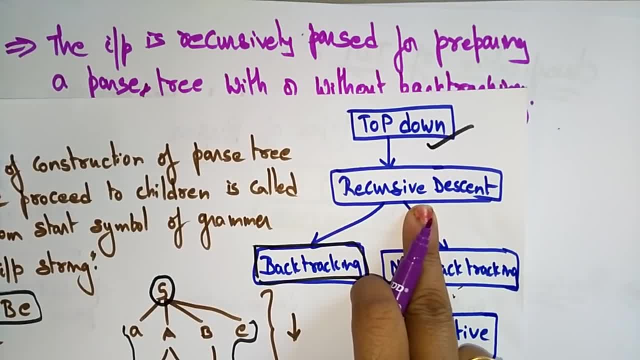 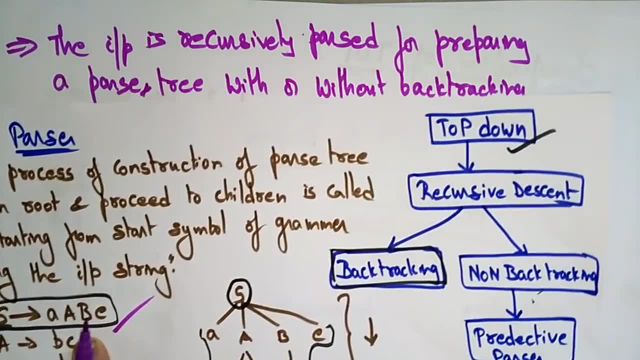 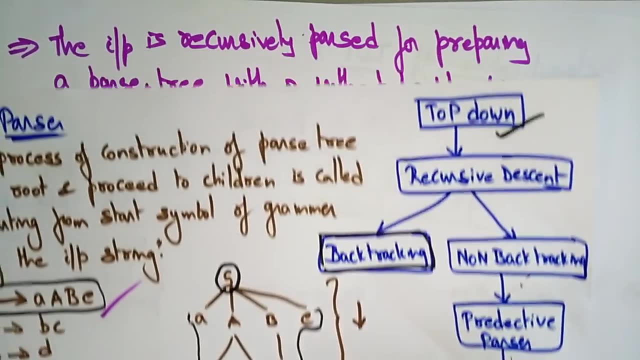 a top-down approach. so here what the main aim of recursive descent: the input is recursively parsed. so whatever the input that we are taking, okay, so this, uh, grammar, whatever the input that we are taking, that input is recursively parsed. for preparing a parse tree. for preparing a parse tree.